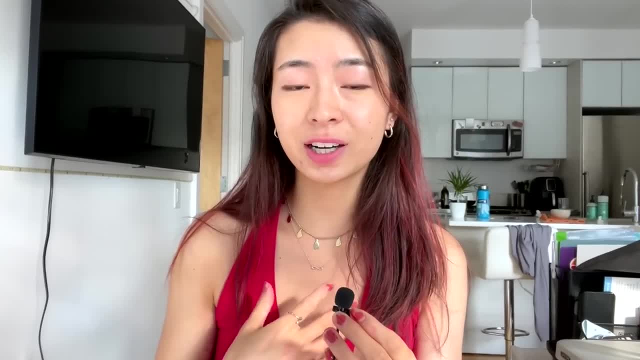 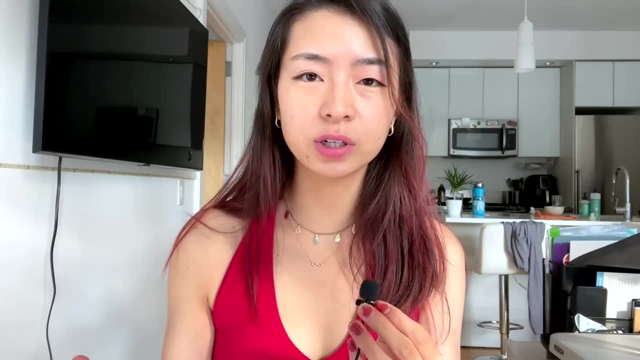 exactly my experience In sixth grade. I was working on problems with three classmates and they just seemed to get it, While to me the math was like a foreign language. I was embarrassed that I was so confused, so I just nodded along, pretending like I was keeping up with them while 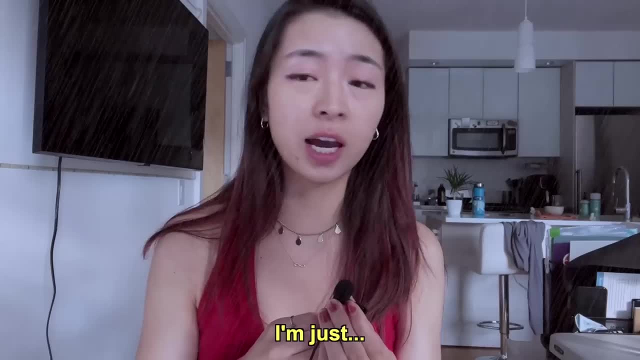 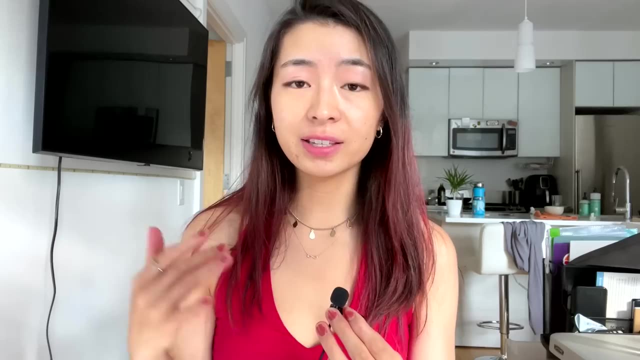 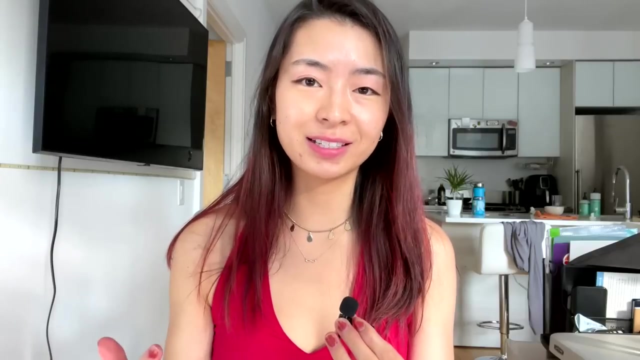 slowly dying inside Like man. this is hopeless. I'm just dumb, I suppose. Later that year, my dad taught me the magic secret of being good at math And starting from eighth grade, I went on to win math competitions, eventually winning a gold medal state level. I was in advanced math classes. 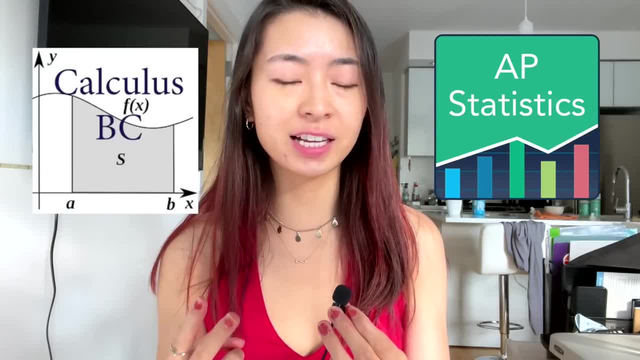 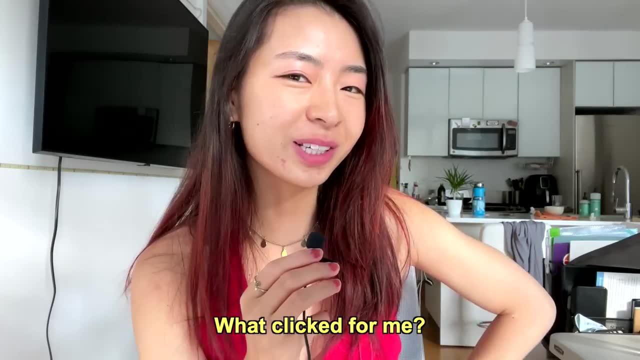 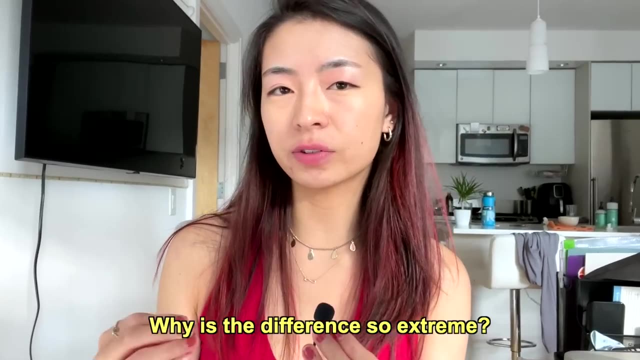 taking both AP, Calc, BC and AP Stats my sophomore year. Now I would rather solve 100 math problems than write one essay. So what clicked for me? Math tends to be the hardest subject for many students, but then the best or easiest for other students. Why is the difference? 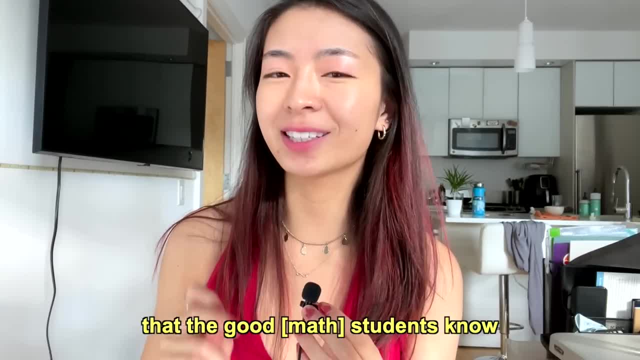 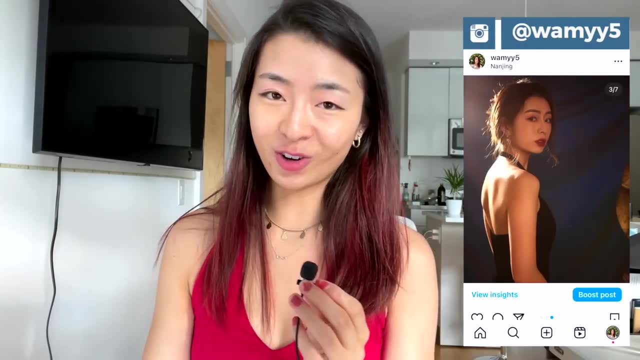 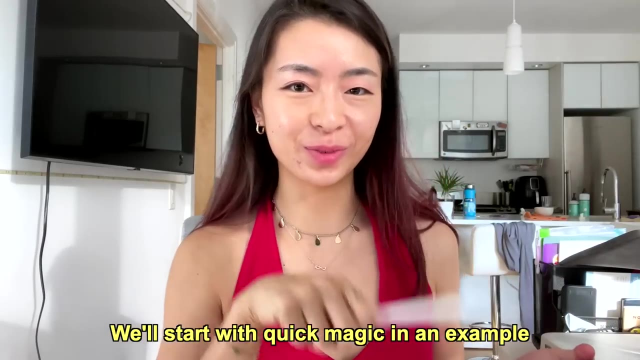 so extreme. There must be a magic secret that the good students know Well there is. So today you'll finally learn the truth behind why you struggle in math And, of course, the solution Warning you might begin to like math. Let's go. We'll start with quick magic in an example: The 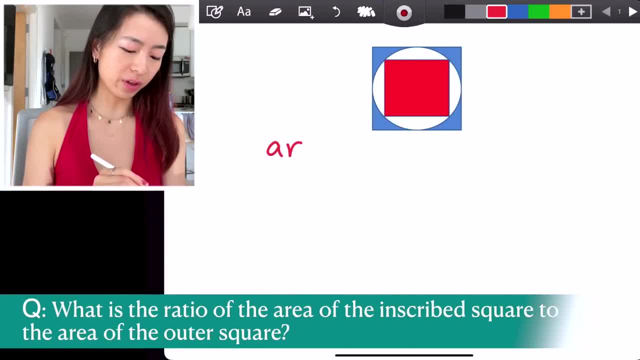 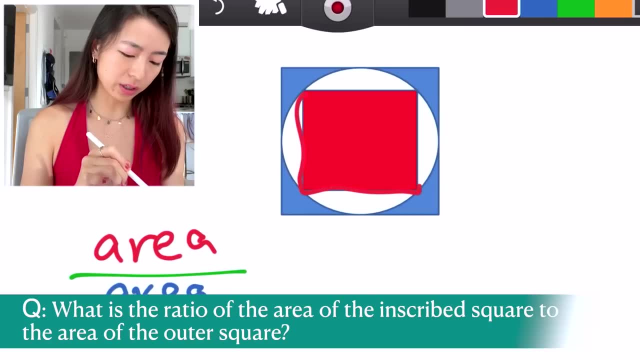 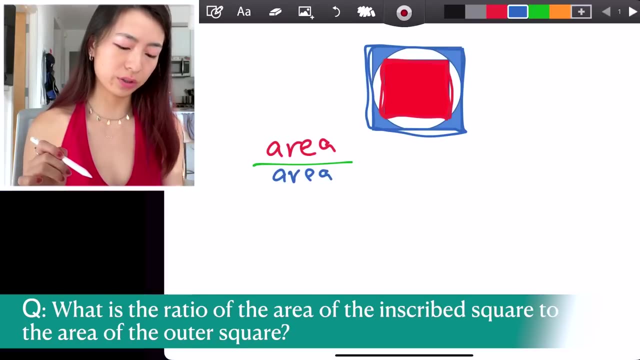 question is: what is erasure Ratio of the area of the red square over the area of the blue square, Basically the area of this divided by the area of everything in these blue borders? Now I'll give you a moment to think. 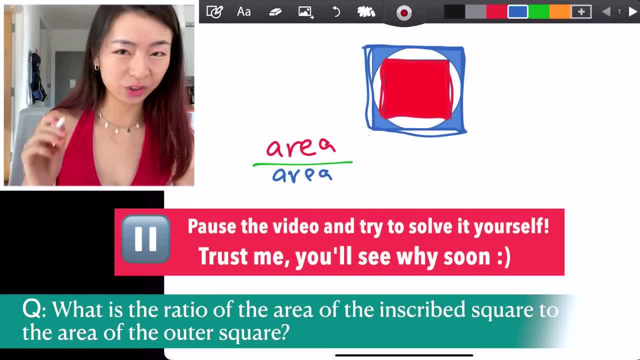 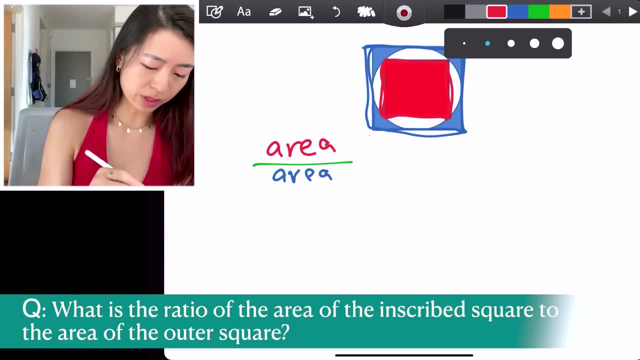 about it, See if you can solve it real quick. That's the fun. Try it, All right, Maybe you tried it, Maybe you didn't. You might have been thinking I'm going to assume you know this side length is. 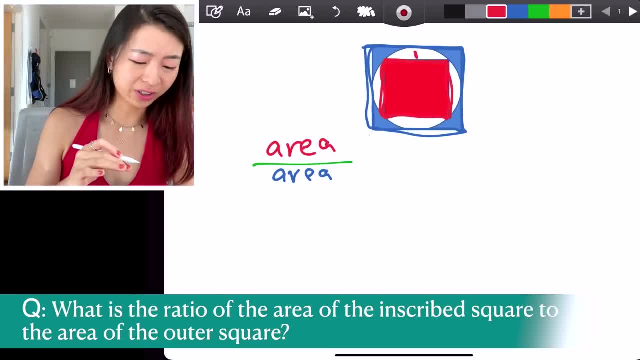 one and then do some circle diameter square relationships to then get the side length of this big square And then, once I get the areas of both squares, I'm just going to do one area divided by the other area. Now, either you thought that or you're like man. I've not seen a problem. 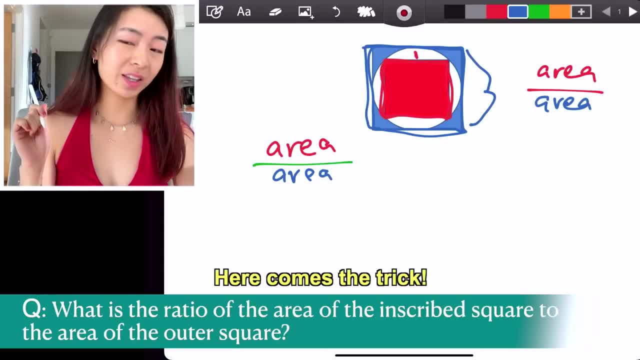 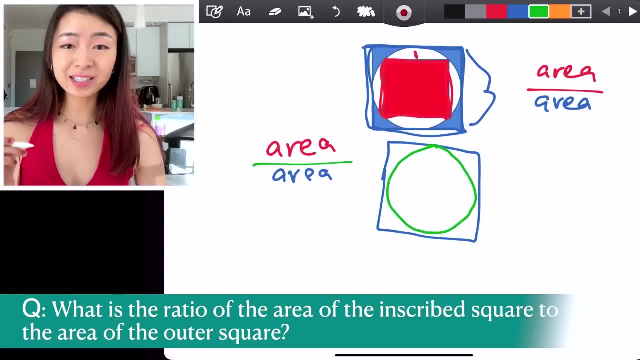 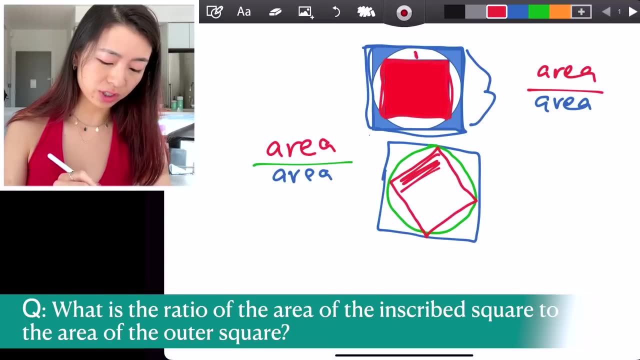 like this anywhere before. I don't know how to solve it. Here comes the trick. I'm going to redraw this shape. Now what if I simply turned the inside square 45 degrees, Like whoa? do you see anything special? 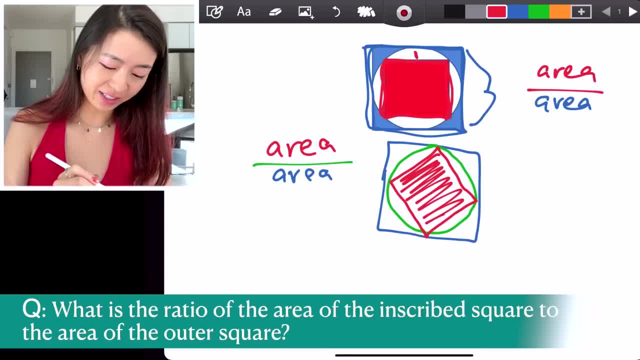 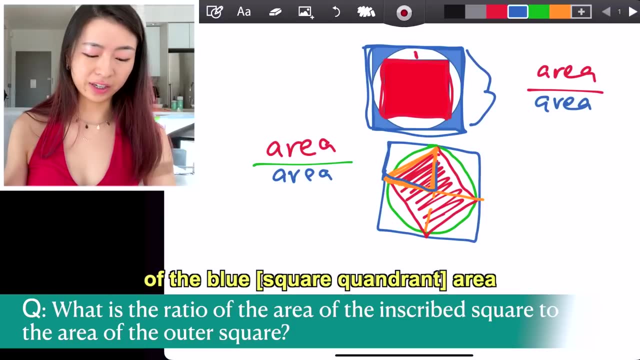 Do you see anything that makes the problem really easy? Yes, indeed. If we cut it up like this, you can see that in each of these four quadrants, the red area is actually half of the blue circle area. So the answer is really easy. You don't need to do any calculations at all. It is. 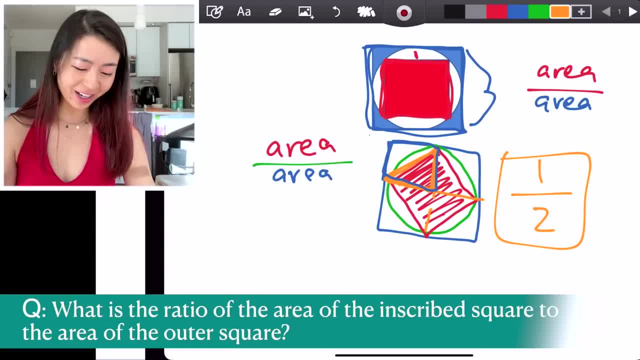 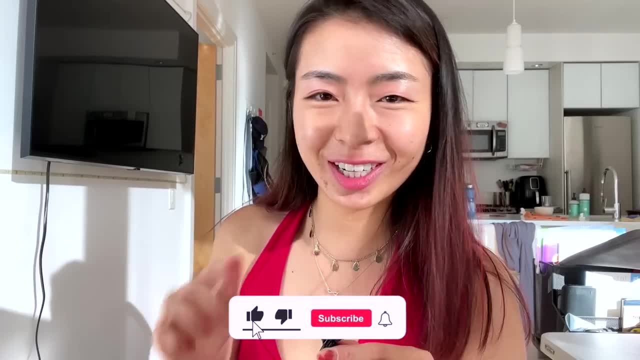 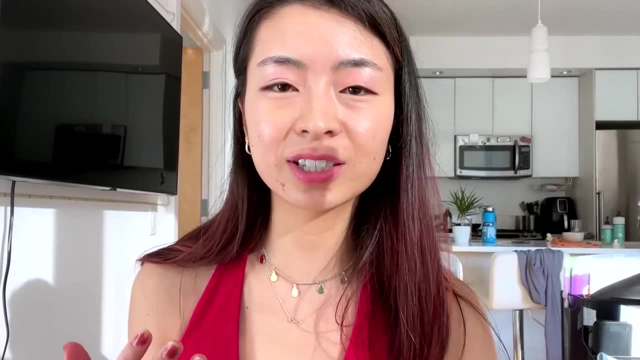 simply one half. Whoa, it's just like magic. This is just like magic. Drop a like right now if you thought that was cool. Come on, guys. That's that's really awesome, right? That's an instance showing that if you have problem solving skills and you're creative in math and understand the 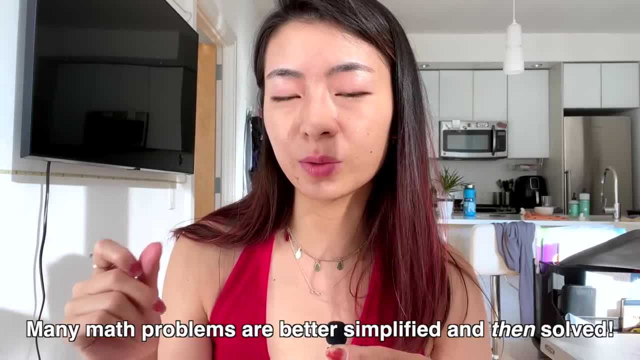 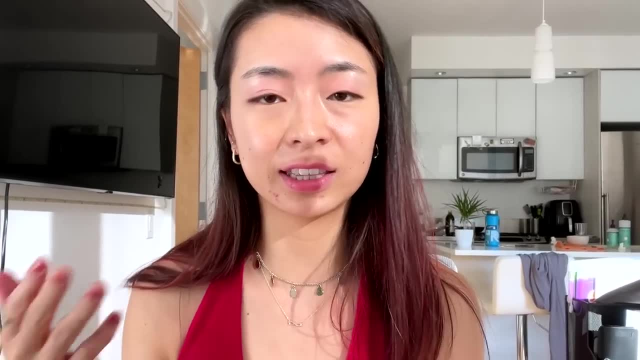 relationships between shapes. you can do one little adjustment or one little flip of the shape And get the answer so much more easily Now. I know your schoolwork probably doesn't look like this question, but here is the headline. It doesn't matter how many formulas you know to solve. 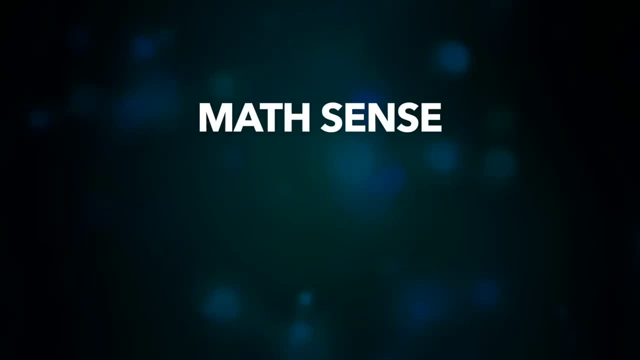 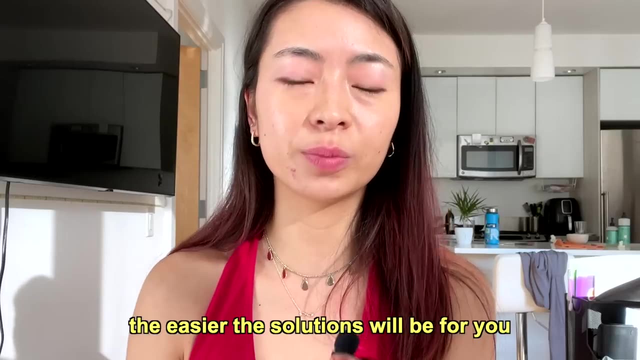 that area problem and other math problems. It's about math sense and problem solving skills. The better your understanding of what math truly is, the easier the solutions will be for you. I'm a private tutor right now for the ACT, SAT and for the math section. I can always get my students up. to make that one of the most important things that they can do. So I'm going to go ahead and take a look at some of the most important things that I can do. So I'm going to go ahead and take a look at some of the most important things that I can do. So I'm going to go ahead and take a look. 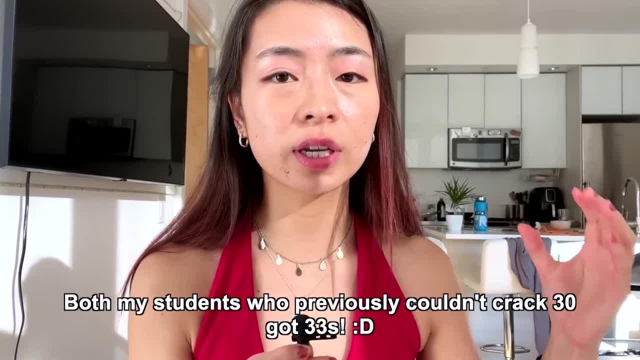 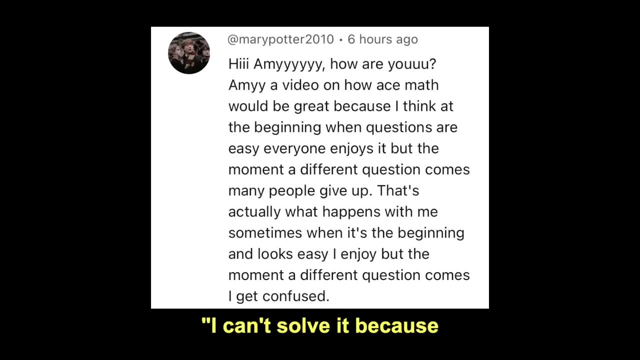 at some of the most important things that I can do. So I'm going to go ahead and take a look at their easiest sections, significantly increasing their scores because of these tricks that I show them, That flip of the mindset I hear all the time. I can't remember the formulas I can't solve. 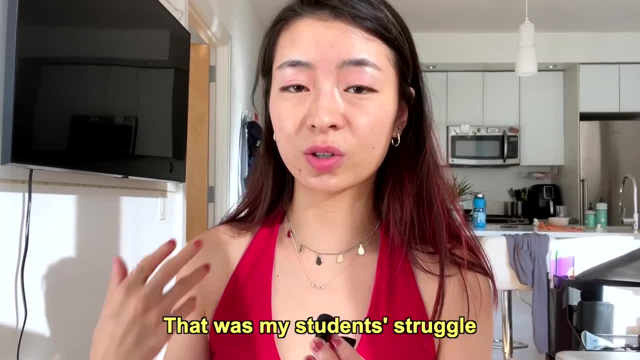 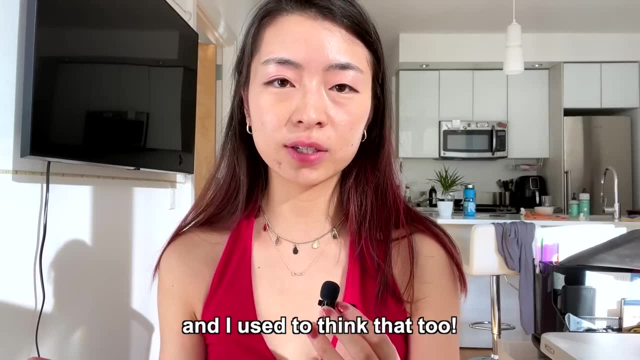 it, because I've never seen a problem like that before. That was my student's struggle and probably yours as well. You think that adding math is just adding more formulas to your brain, more tools to your toolbox. But let me ask you this: If you were a construction worker who 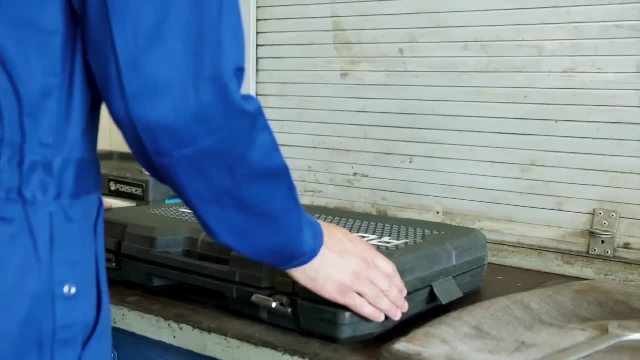 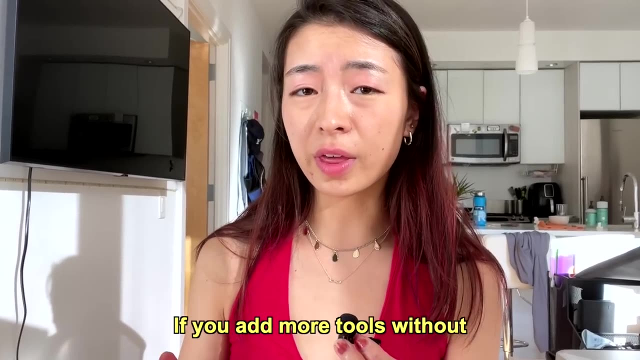 wanted to improve. what would be more helpful: Relying on adding more tools to your toolbox or increasing your actual skills as a construction worker? If you add more tools without really knowing how to use them, you're just going to get more and more overwhelmed as a construction. 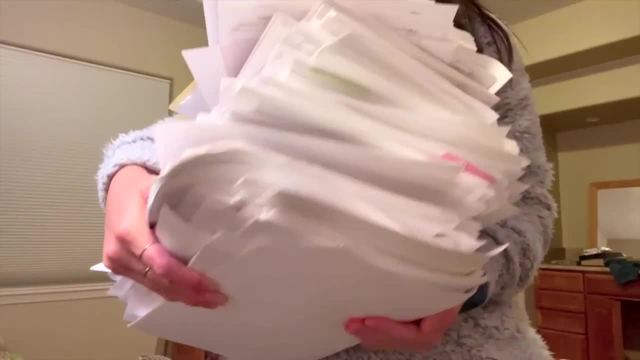 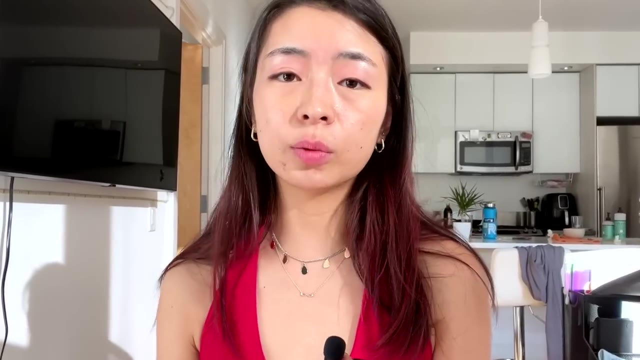 worker Like you won't be able to get anything done. You'll just be piled under this accumulating weight of all these new things you have to remember and use, Just like in math. if you're not improving your real math skills, you'll fall more and more behind because there's so much more. 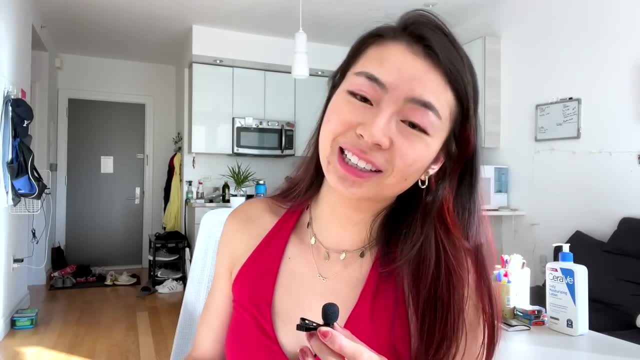 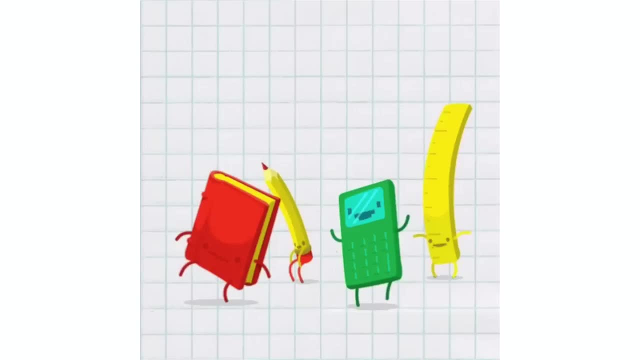 and more to memorize, But when you really learn and understand, you solve more problems with less effort Like. no wonder those math students find it their best subject. Using your math toolkit becomes easy when you don't have to think hard about what to use, when and how to use. 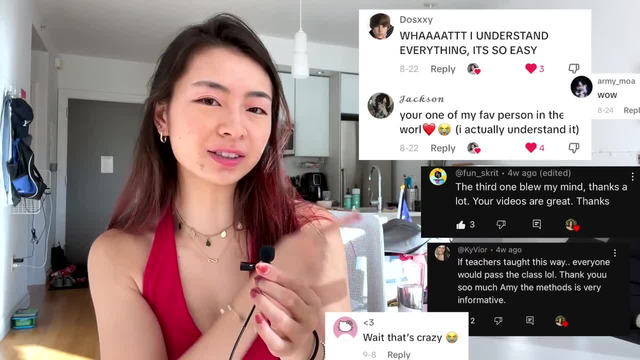 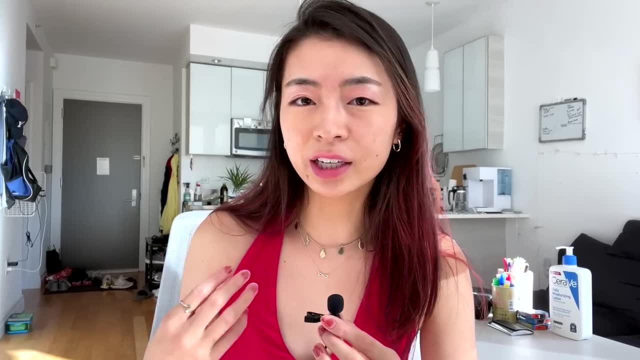 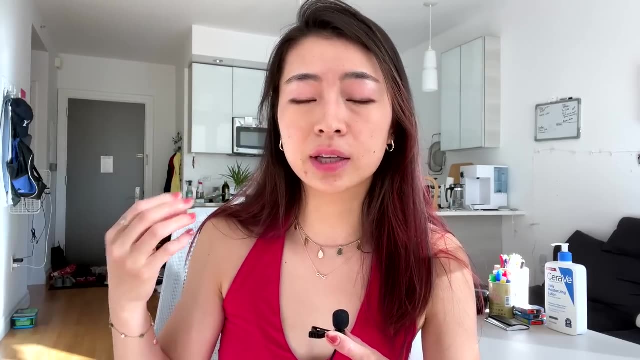 it And at the end it is like magic. Like check out these comments from students who watched my ACT, SAT, math tricks video. I didn't have to try and remember those tricks from all those years since I took the ACT and SAT so long ago. I just had that math sense. that's always there, that's. 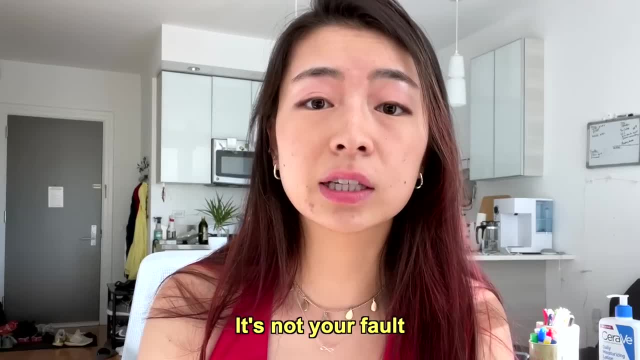 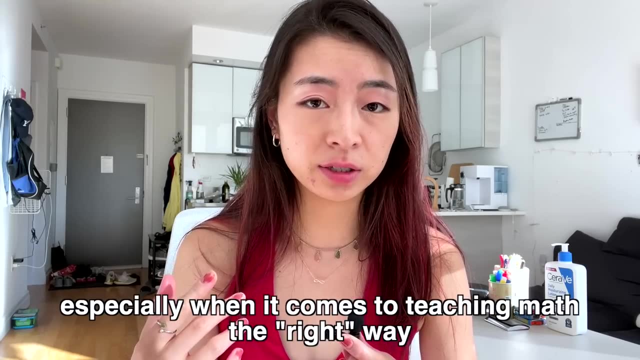 going to help me solve any problem that comes my way. The truth is, it's not your fault. I'm sorry, but there are many subpar teachers out there. I've seen it with my own eyes. One of my students right now tells me that his teacher just writes some things on the board, sits back and goes learn it. 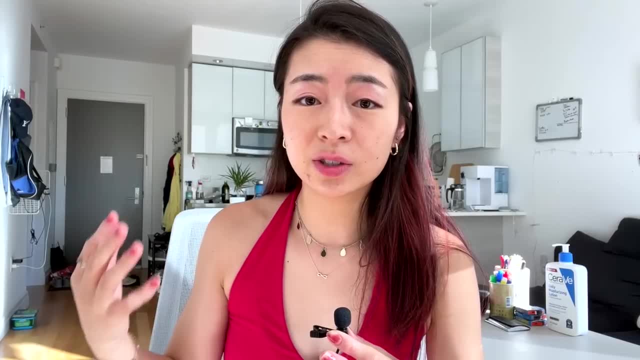 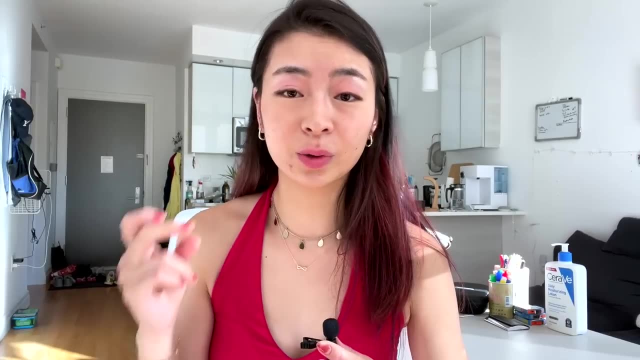 and then gives him the test. That is not math, guys. So really don't feel bad if you have been living your life so far not knowing that this is the real way to get good at math. Another quick example before we go into the solution. 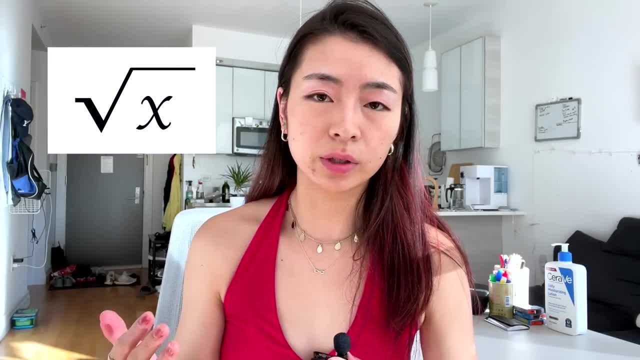 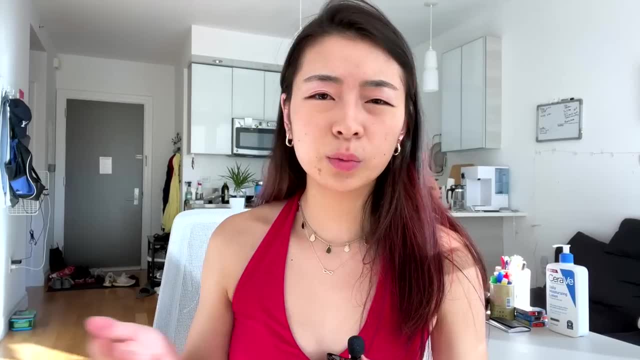 Think about square roots. If you were just trying to memorize square roots, like you learned that square root of 25 is 5, then if someone asks you what is the square root of 36? You wouldn't know because you never learned it. It's not in your memory. On the flip side, if you knew what the 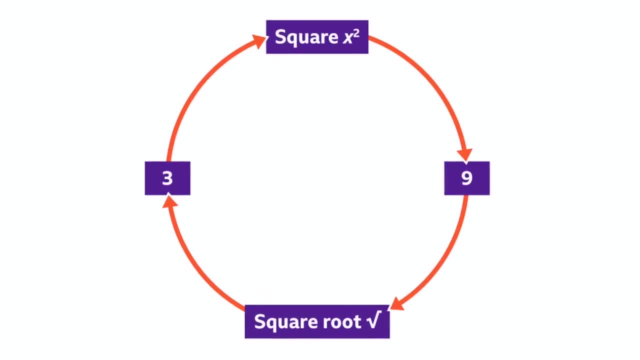 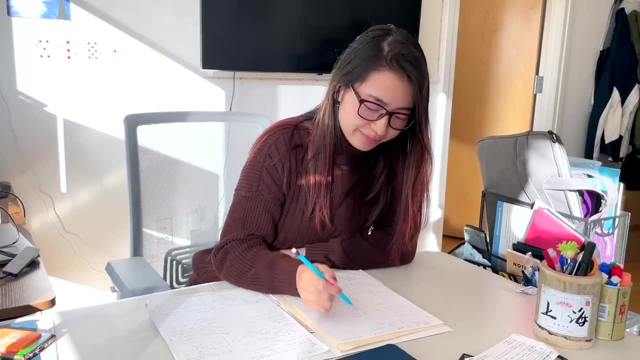 square root actually means as the inverse of squaring a number. then you know what the square root of 36 is. Imagine the next time you take your math test and all the solutions just come to you. Here's how to make that happen. 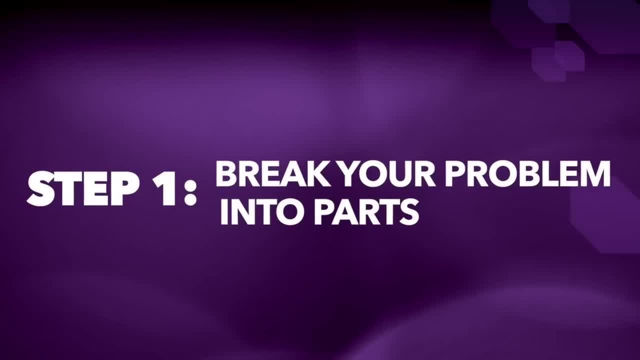 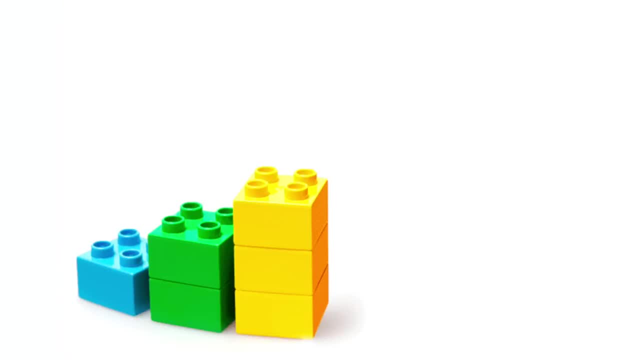 In a three-part solution. you should do this while practicing math Number one. take your math problem and break it into parts. Often we don't even realize that we don't actually understand the little foundations behind the bigger, more complex math problem. So, for example, if you have a big 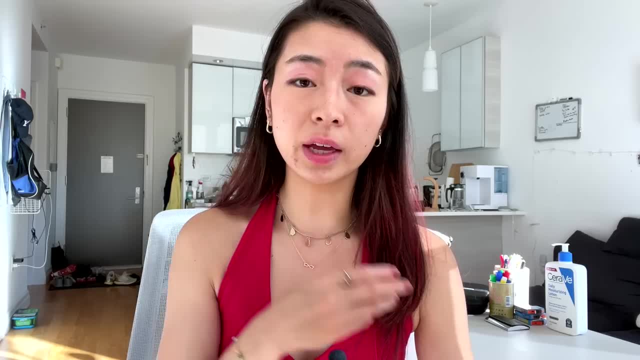 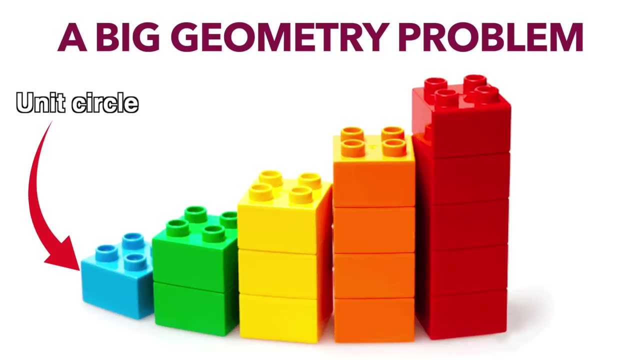 geometry problem and using the unit circle as part of it, then the concept unit circle would be a piece of that math problem. So you would break that math problem into unit circle, then maybe algebra operations, whatever you want to call it. So if you have a big geometry problem and you 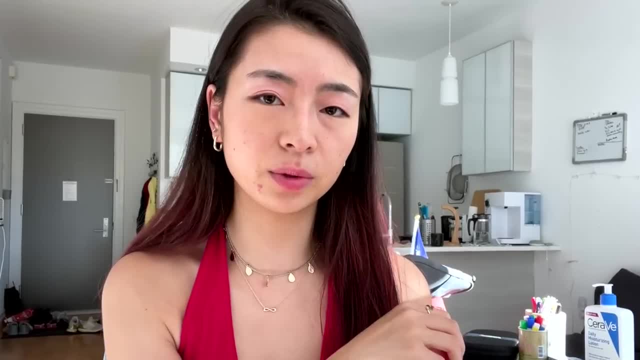 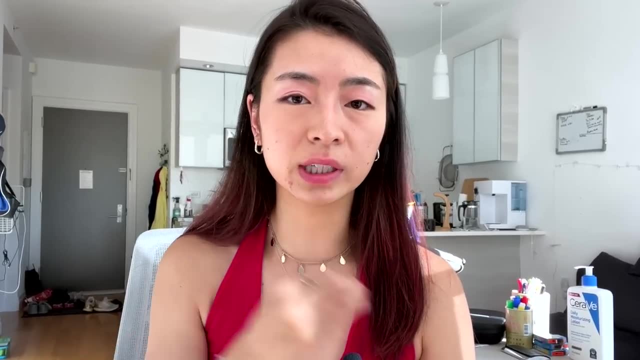 don't know how to solve it, then you can use the unit circle as part of that math problem. Number two: once you have your math problem broken into those foundational parts and you know the tool you need for each part, then review the tool you use for each part. So in that unit circle, 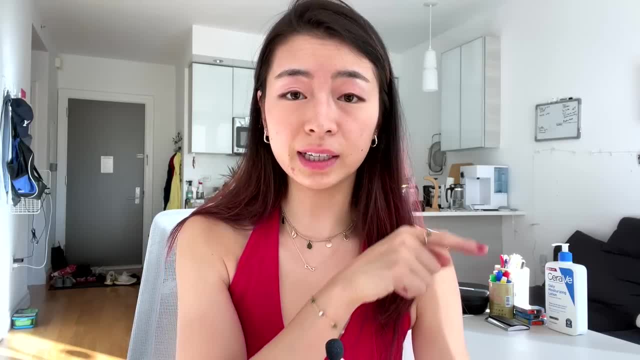 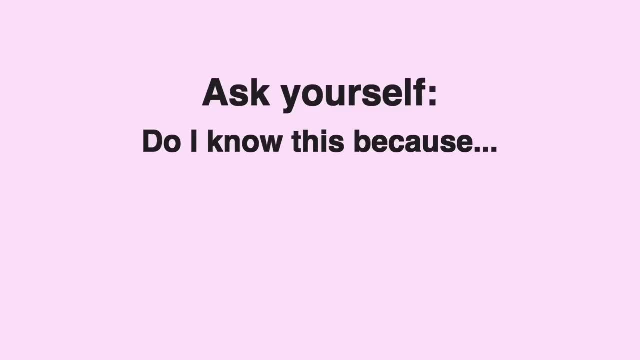 example, the tool or concepts you might need are what the xy coordinates are all around that circle and what the radians are around that circle. Ask yourself: do I know this because I'm memorizing it, or do I know it because I'm memorizing it? And if you do, then you're going to be able to figure out. 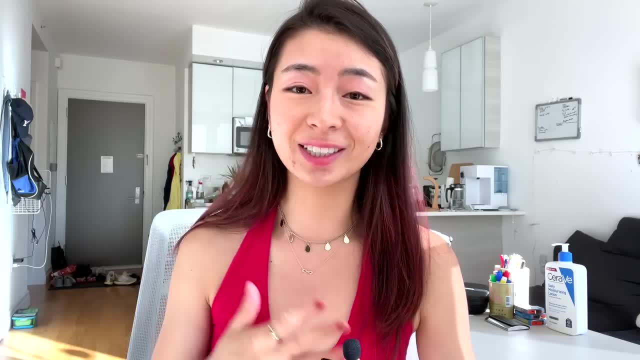 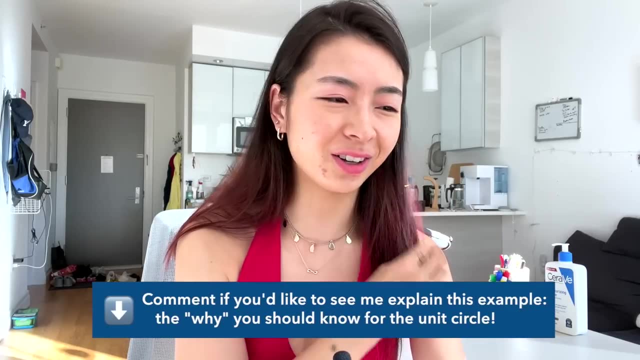 if you know it, because I understand it. If it is the former and you don't actually understand it, then watch videos on that concept and the origin, the reason behind why all of those numbers are around the unit circle. Khan Academy and YouTube both have excellent resources, so just watch as. 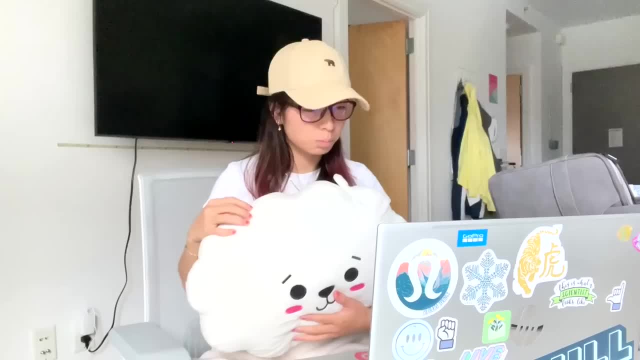 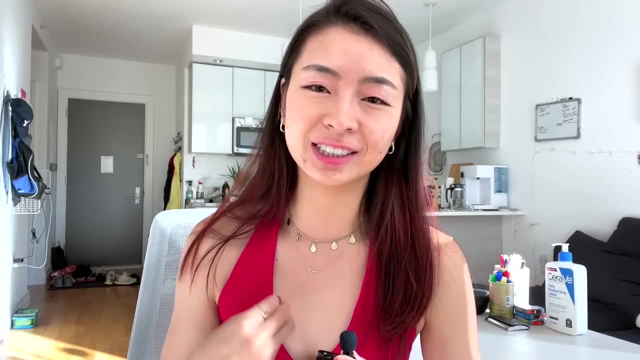 many, as you need to understand it, Maybe even do some practice problems. Repeat this process for each foundational part of your original problem so that you actually understand and have the fundamentals good again. If you don't know how to solve it, then you're going to have to do it again. 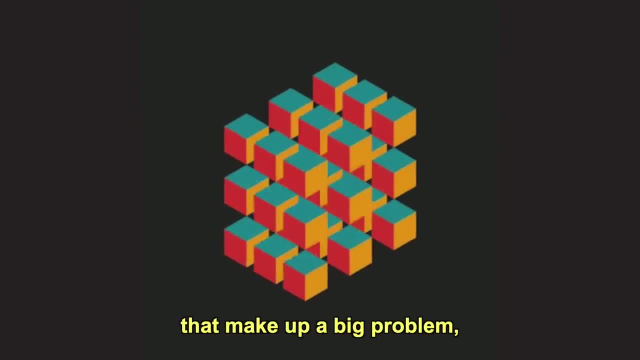 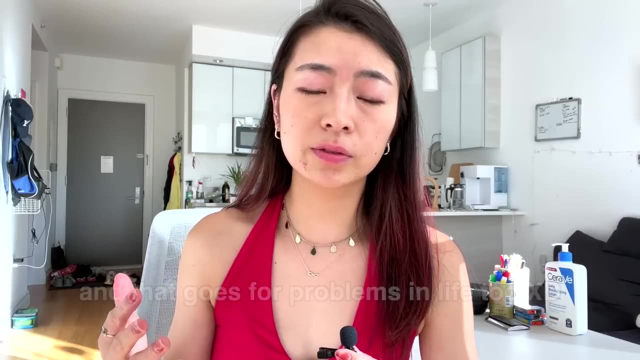 If you don't feel confident and strong in the little concepts that make up a big problem, then every big problem and the bigger and bigger problems that come after that will be even harder. This works for basically any math problem And I know I used the unit circle, but the reason I 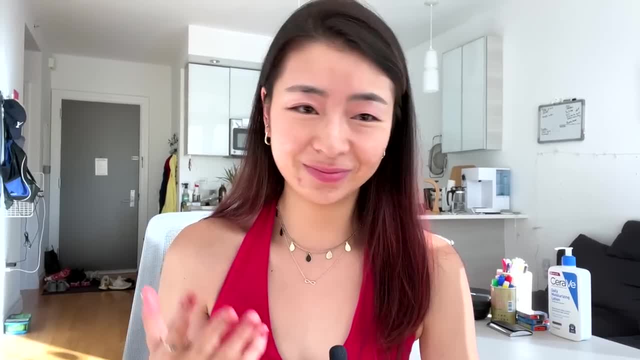 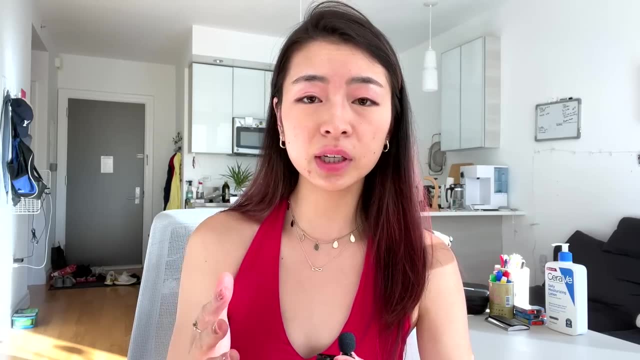 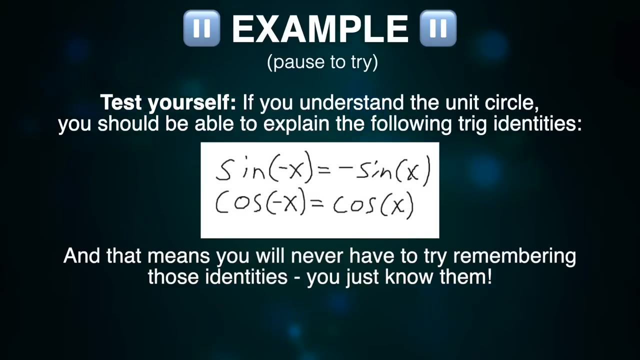 bring that up is because me, after like eight, many years of not using the unit circle or even seeing it in front of me, if you gave me a blank unit circle, I would be able to fill in all of those numbers right now. That's the power of understanding and not memorizing, And that's also why I can take the ACT- math live. 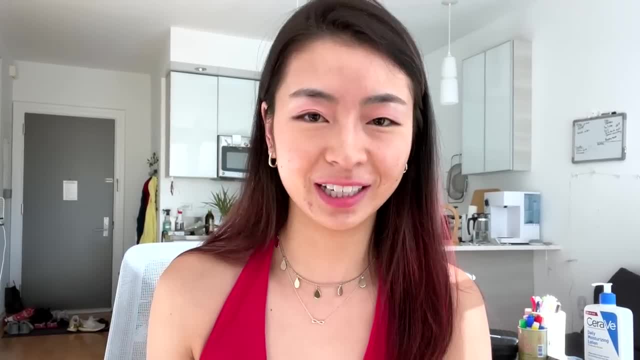 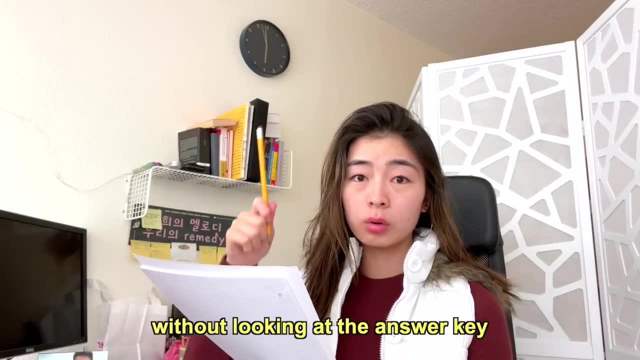 and get a 36 on it even without any preparation right now. Number three: solving that initial big math problem. Try to solve it on your own from scratch, without looking at the answer key. Even when you do get to a problem and feel stuck, don't look at. 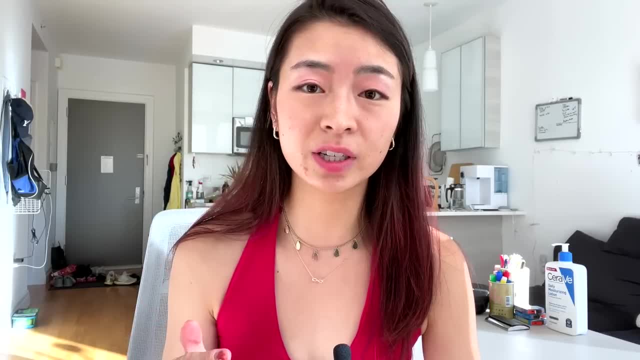 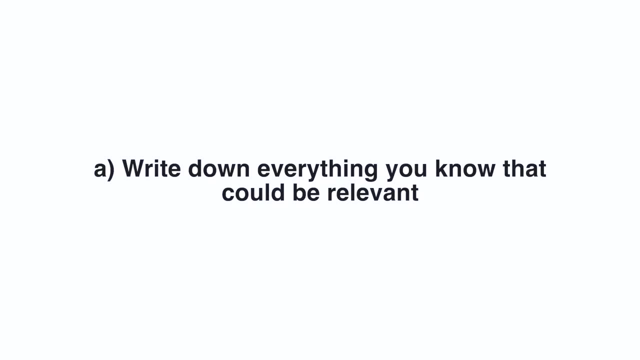 the answer key. yet I know it's really tempting because the solution's right there in the back of the book. But don't do it, Stop. Stop it First. write down everything you know about the problem in front of you, If like an ACT problem. 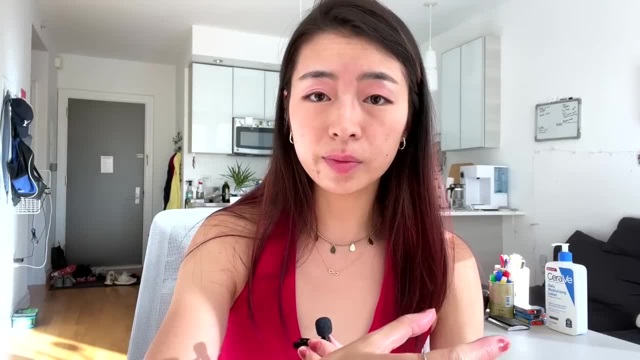 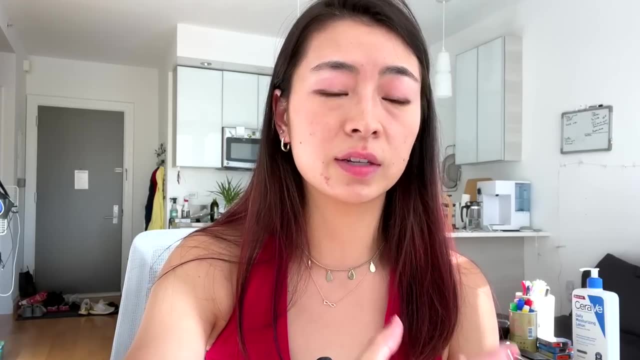 it asks you: how do you make this number even? The term there is even. So think back to everything you know about even numbers. When I did this with my student and my student said an even number is divisible by two, he immediately knew how to solve the problem. At first, my student was stuck. Then 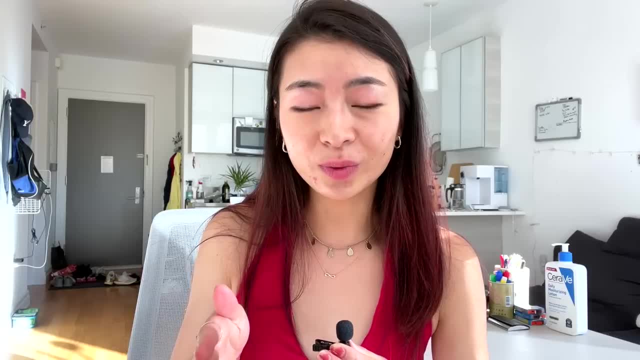 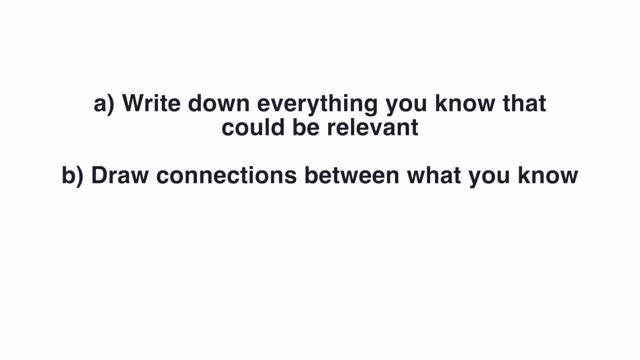 I simply asked him: what do you know about, even numbers? He told me, and then he knew how to solve it on his own. After you think about everything you know about that one problem, try and draw connections between those things. I encourage you to write that down. This is like: 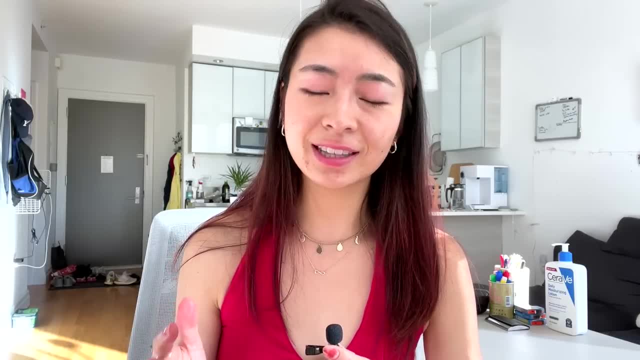 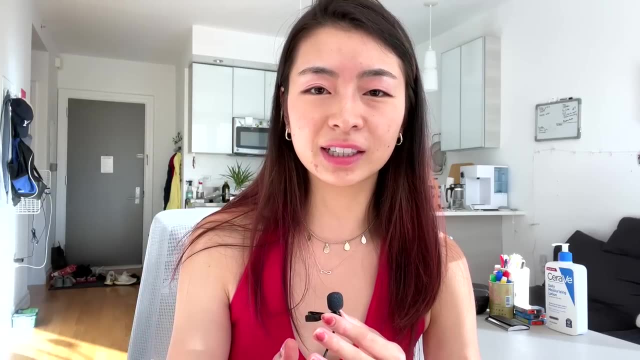 your attempt at a solution. Think about it for a few more minutes and then, if you're still stuck, yes, now. go into the answer key Now. when you're looking at the solution, compare it to your initial thinking and see how similar or how different it might be. 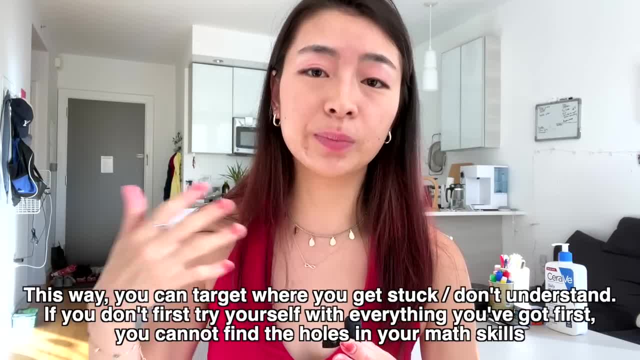 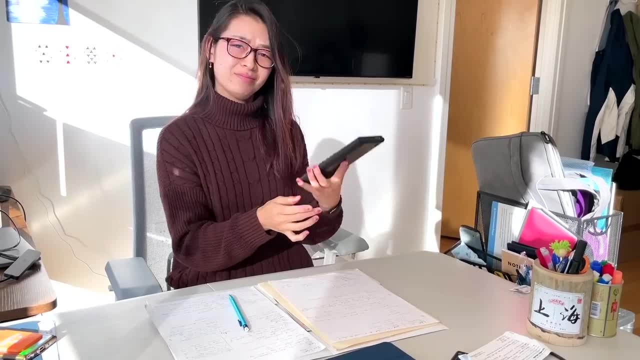 This is where the learning and problem-solving ability gets built over time. This last step is so, so important, because if you only look at the solutions instead of trying the problem yourself as much as you can first, you won't build problem-solving skills. The real world doesn't just. 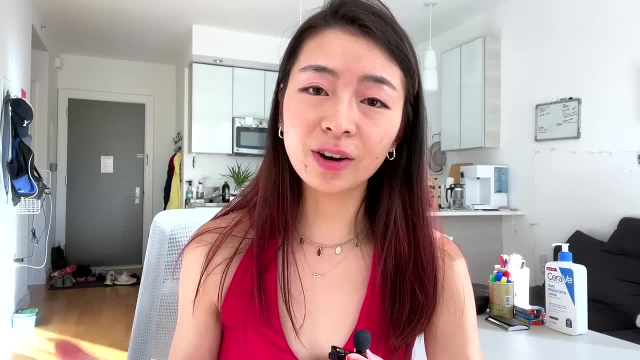 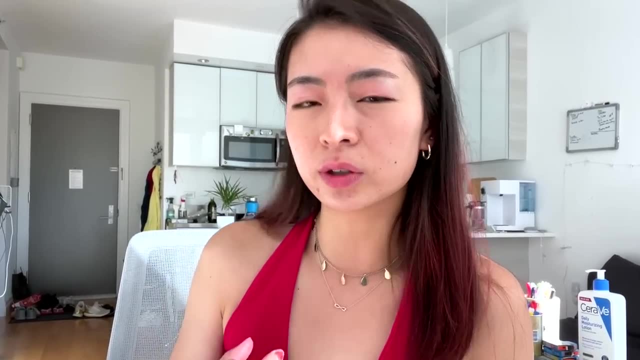 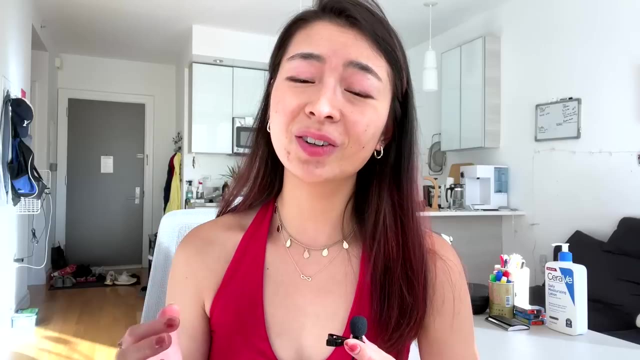 hand you solutions on a silver platter. You'll have to figure them out on the job, otherwise your boss is gonna hate you, man. That's why this approach of understanding and attitude of wanting to build your math skills will set you up for success in the real world too. I know it's going. 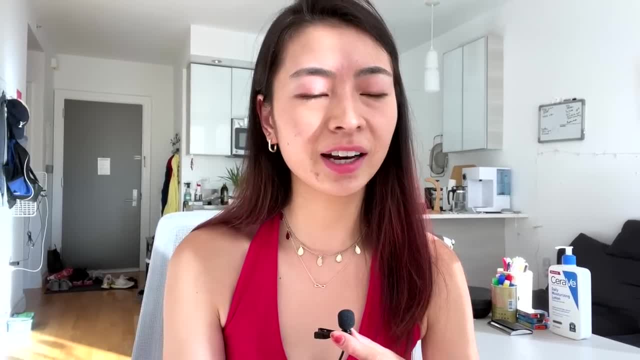 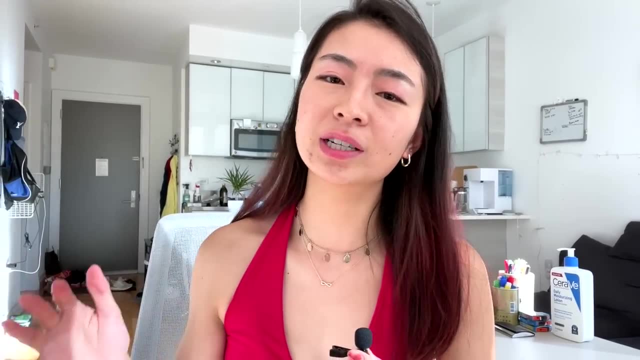 to be hard to flip the switch. at the beginning, When I was getting taught by my dad, I was like this is taking so long. Why are you explaining all these things? I just need to get the problem done. All that upfront effort will pay off so much in the long run. Trust me from my experience. 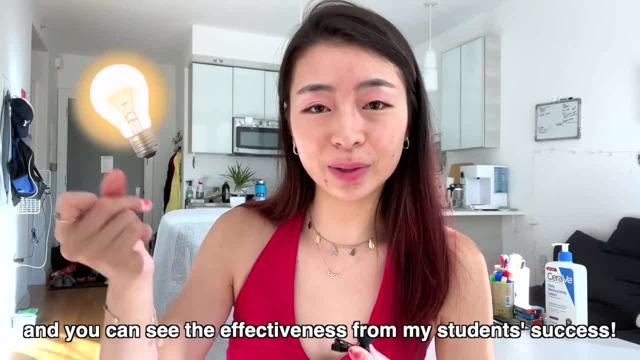 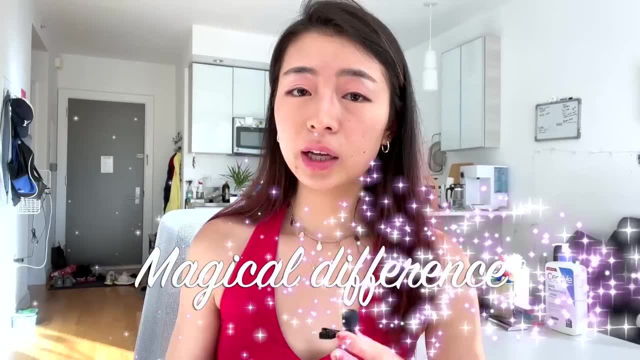